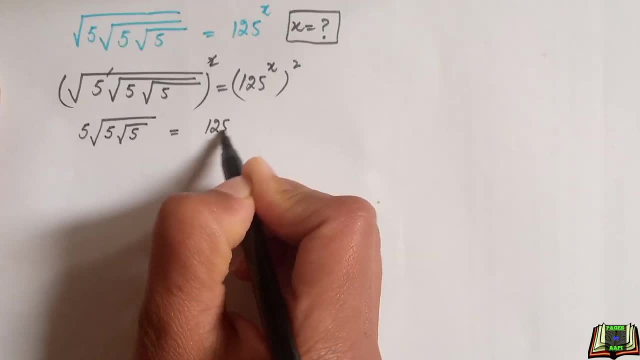 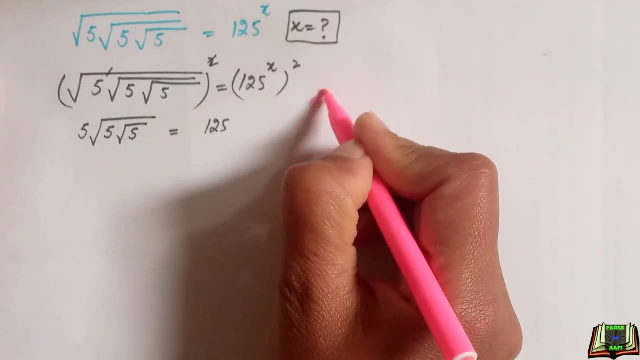 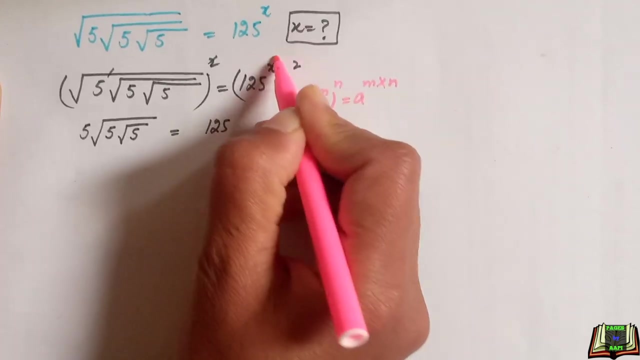 is equal to 125 and these two powers are going to multiply because we are going to use allow for power power of a power rule That says if a raised to the power m raised to the power n, then we can multiply the powers m times n. So here we are going to multiply. 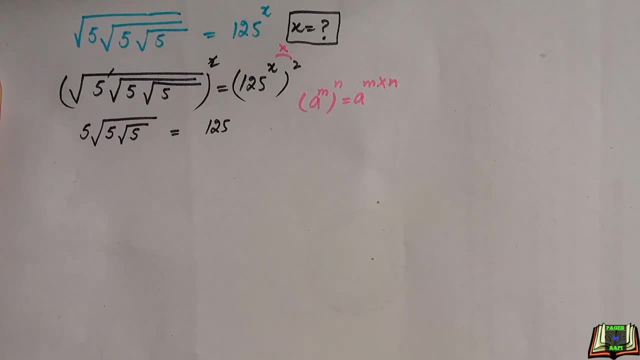 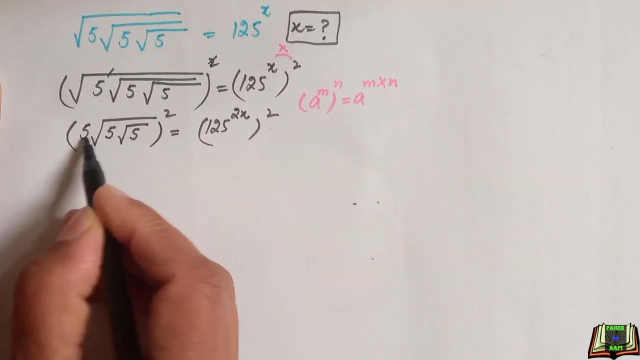 these two powers: 125 raised to the power 2x. Once again, we will take the square of this equation on both sides. So this is equal to 5 to the power 2 and this square and root of 5 times, 5 times square root of 5 is equal to 125 raised to the power. These two powers. 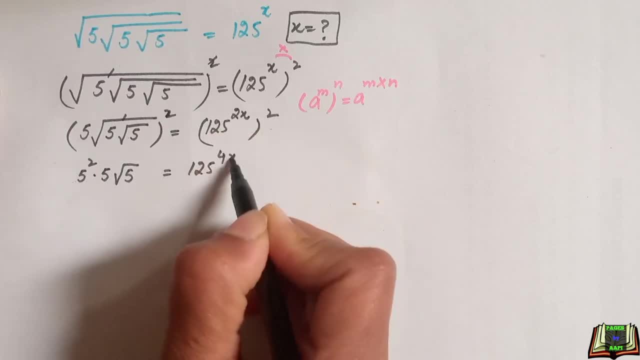 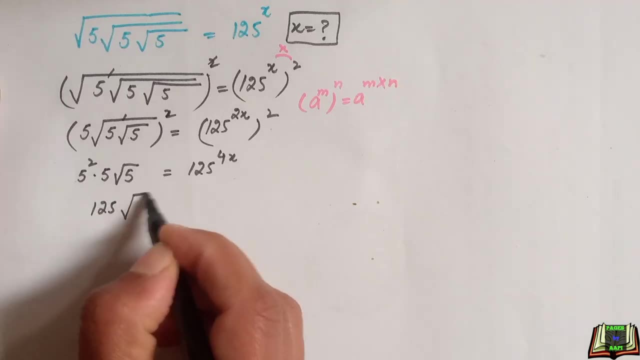 are going to multiply once again 4x. This is equal to 5 to the power. 2 is 25 times 5 is 125. square root of 5 is equal to 125 raised to power 4x. At this stage, we are going to: 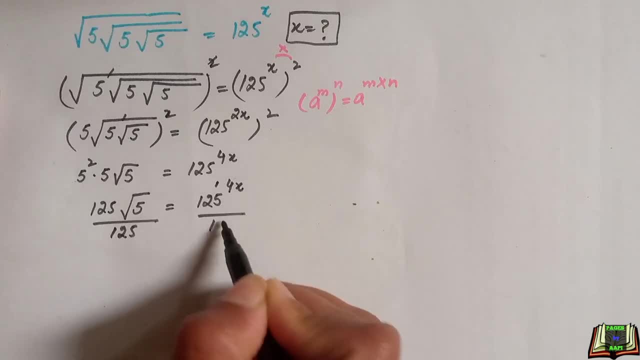 multiply both sides by 125.. So this and this cancel out, square root of 5 is equal to here. we are going to use another law of exponent which says: if a raised to the power m divided by 8 raised to the power n, then we can subtract the powers m minus n. Similarly, 125 raised. 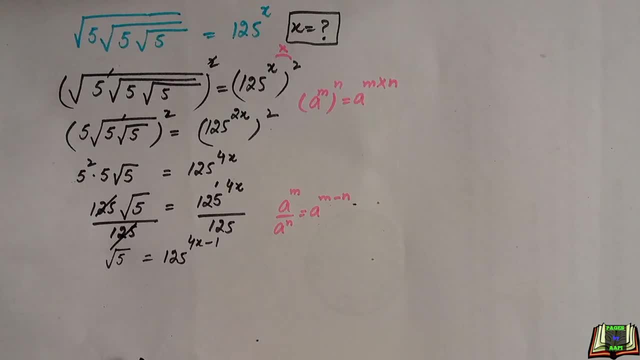 to the power 4x minus 1.. After taking square of this equation, on both sides this is equal to 5 and right hand side 125,. 2 is going to multiply by 4x minus 1, which is equal to 125. raised to power 4 times 2 is 8. 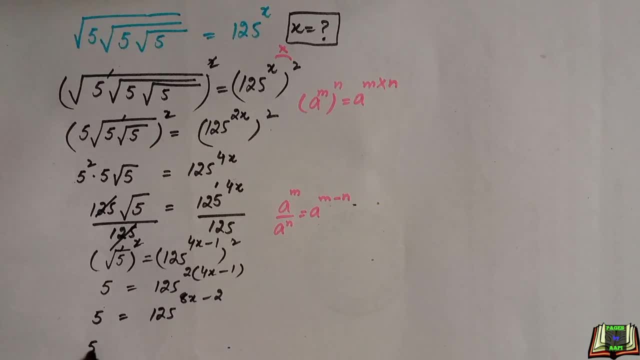 x minus 2, 1 time is 2.. 5 is equal to this. 125 is equal to 5 times 5 times 5, which is equal to 5 raised to power 3.. So we are going to replace 125 by 5 raised to power 3 times 8x minus 2.. 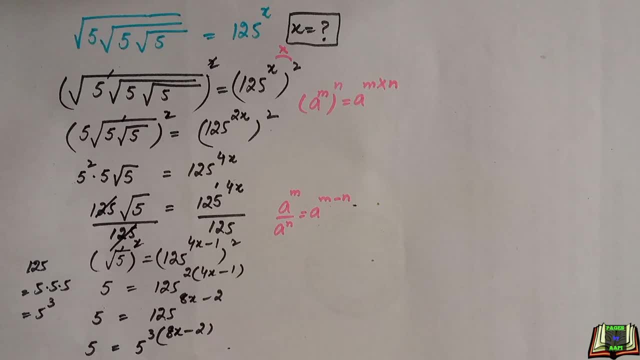 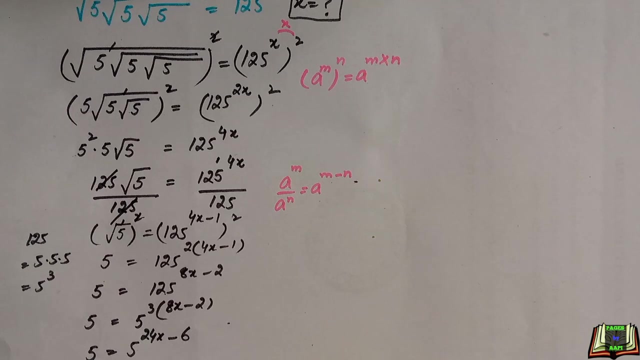 In the next step we are going to multiply: 5 is equal to 5. raised to power 8 times 3 is 24. x minus 3 times 2 is 6.. Now, as bases are same, so we can equate the powers. This left hand side, 5. 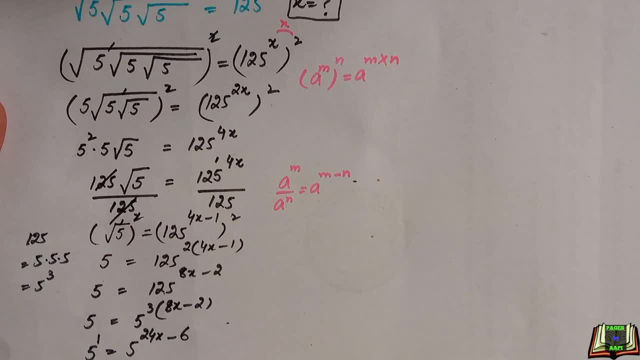 is basically 5 raised to the power. 1 is equal to 5 raised to power, 24 x minus 6.. So we can write it as: 24 x minus 6 is equal to 1.. We are going to add 6 on both sides. This is equal to 24 x. This 6 and 6 cancel out is equal. 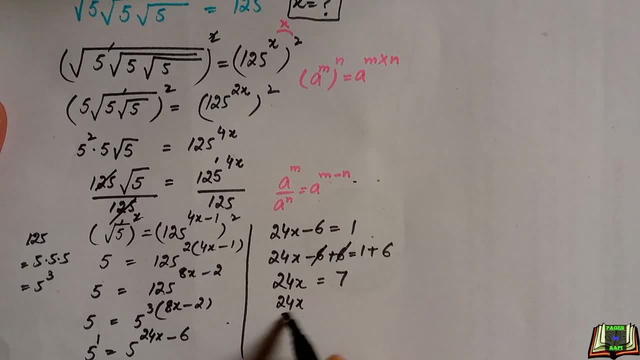 to 7.. Now we are going to divide both sides by 24.. So this 24 and 24 cancel out. We are left with x is equal to 7 over 24.. This is the final answer which is required in this question. 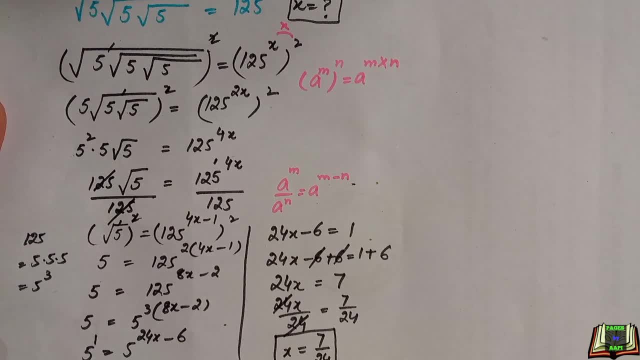 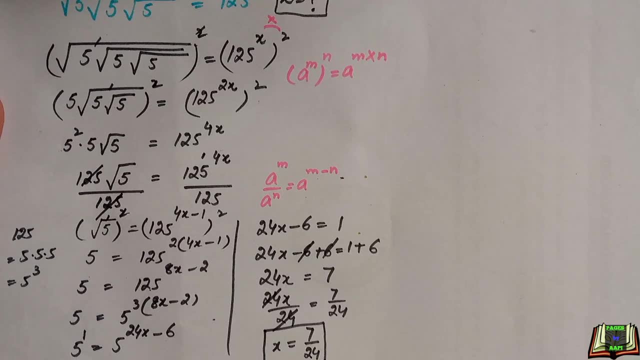 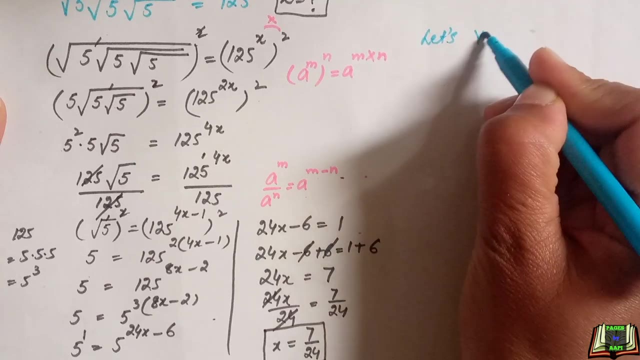 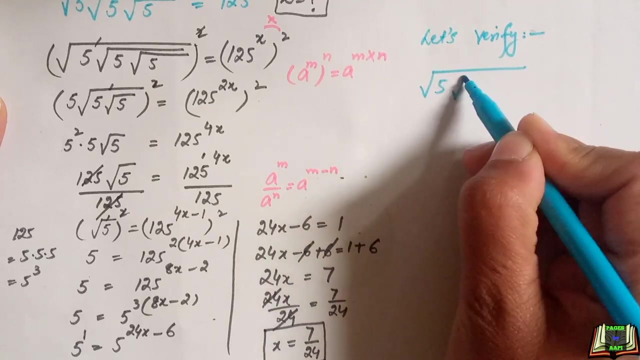 But we are going to verify our answer, that it is the correct answer or not. So let's verify our answer by putting the value of x in question. Let's verify. And the question is: square root of 5. square root of 5. square root of 5 is equal to 125 raised to power x. 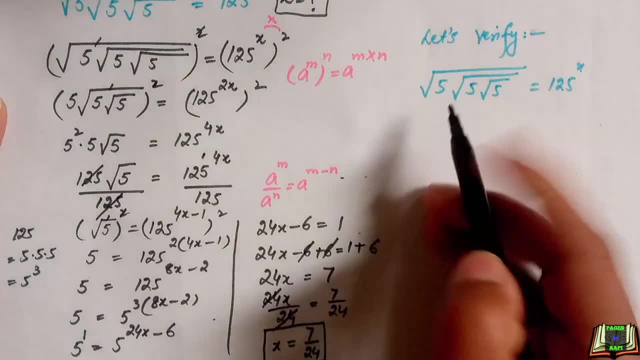 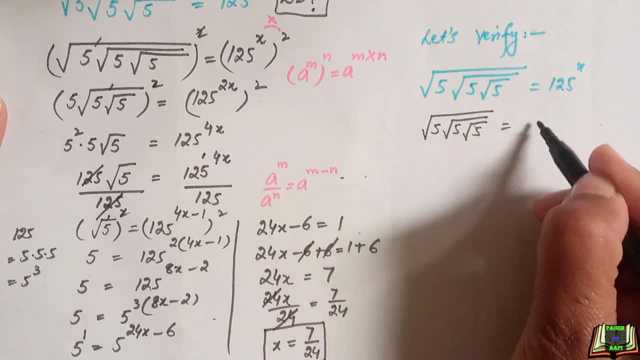 And we know the value of x. Now we are going to put the value of x in this question. Left hand side will be written as it is And this 125 raised to power 7 over 24.. We can write this as square root. 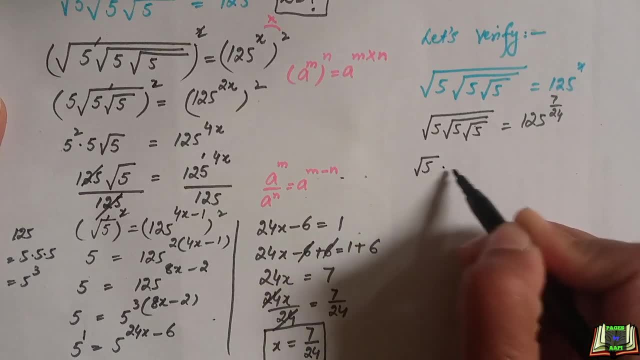 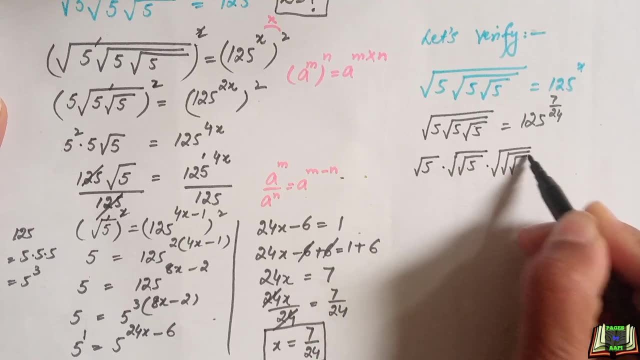 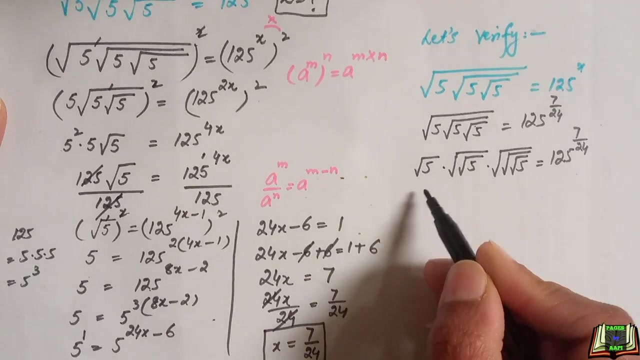 of 5 times square root of square root, of 5 times square root of square root of square root. 5 is equal to right hand side as it is, We know the value of square root. This is equal to 1 over 2 times 5, raised to power. 1 over 2 times 1 over 2 times 5 raised to power 1. 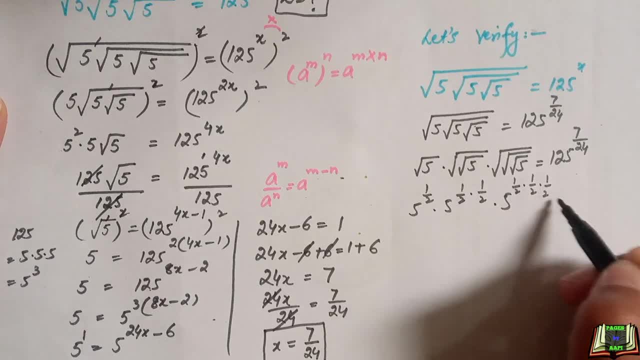 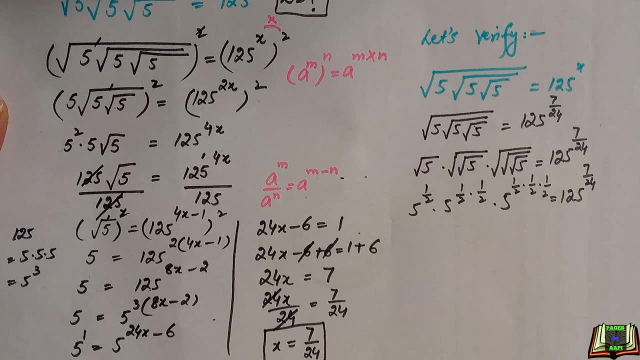 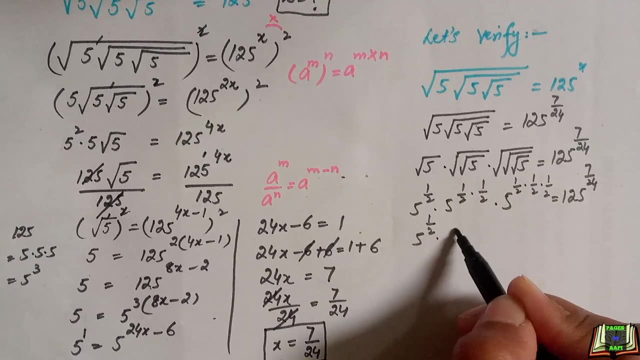 over 2 times 1 over 2 times 1 over 2 is equal to 125 raised to power 7 over 24.. Now we are going to write this as square root of 5: 5 raised to the power 1 over 2, as it is times 5 raised to the power 1 over 4 times 5 raised to the power 1 over 8.. 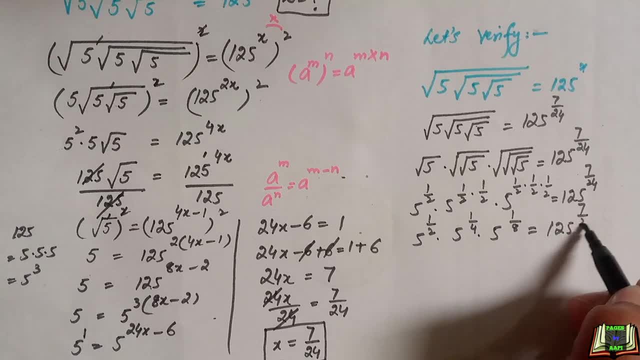 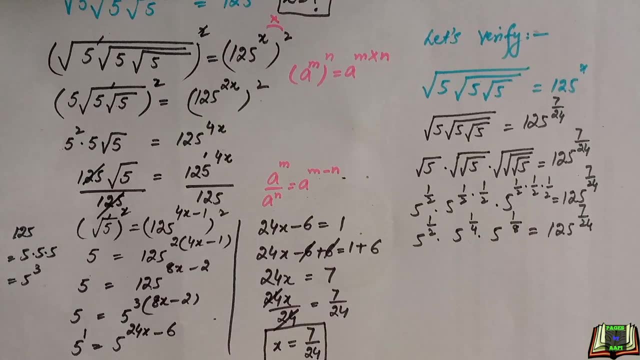 As bases are same. so we are going to add the powers. We are going to use another law of exponent. That law of exponent says: if a raised to power m times a raised to power n, then we can add these bars m plus n, so 5 raised to the power 1 over 2 plus 1 over 4 plus 1 over 8. 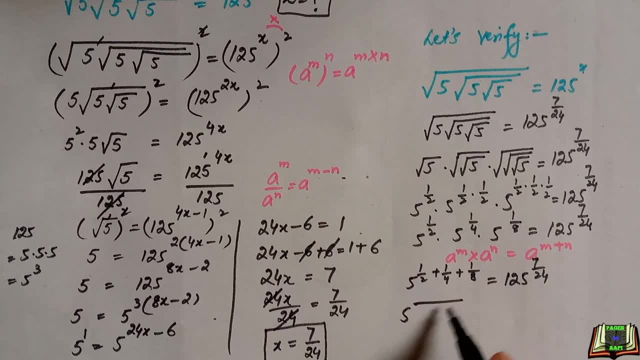 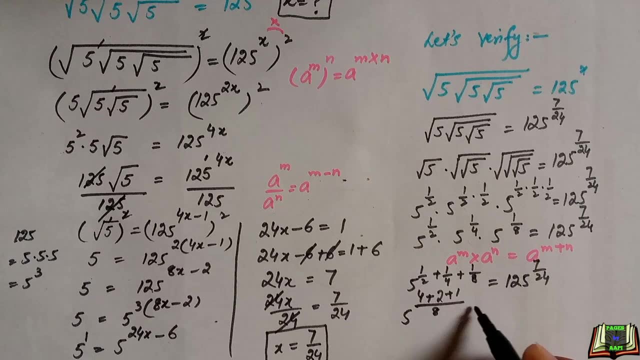 in the next step we are going to take, the lcm. lcm is 8. 2. 4 time is 8. 4 1 time is 4. 4, 2 time 8: 2 1 time is 2 plus 1, 5. raised to the power, 4 plus 2, 6 plus 1, 7 over 8 is equal to: we can: 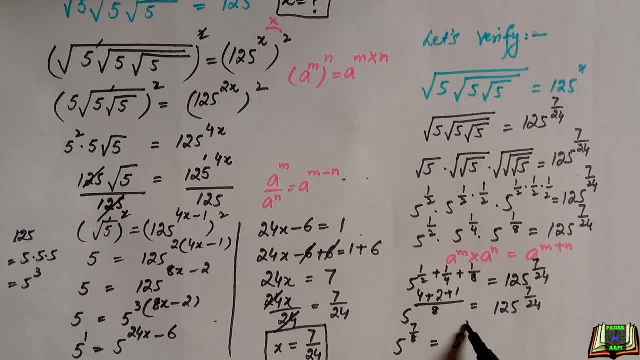 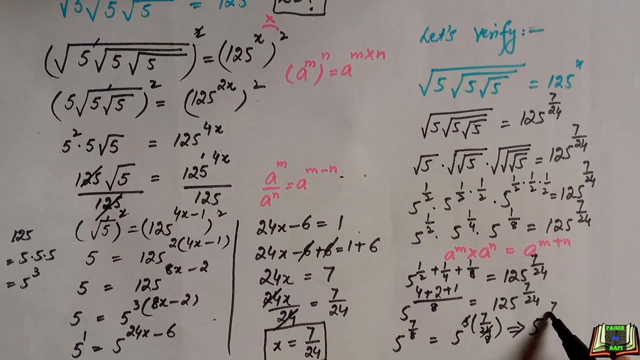 write 125 as 5 raised to the power 3 times 7 over 24. now this can be cancelled out: 3: 1 time is 3 and 3- 8 time is 24.. now we can see that 5 raised to power 7 over 8 is equal to 5 raised to power 7 over 8. it means: 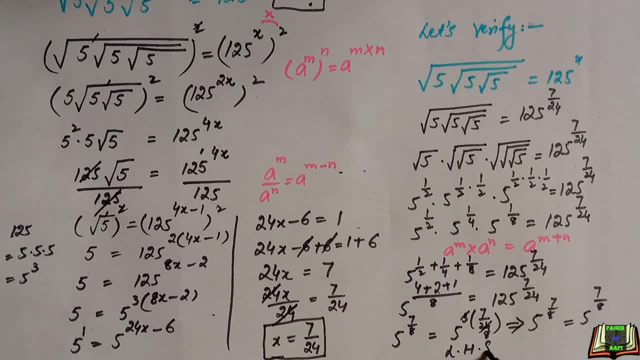 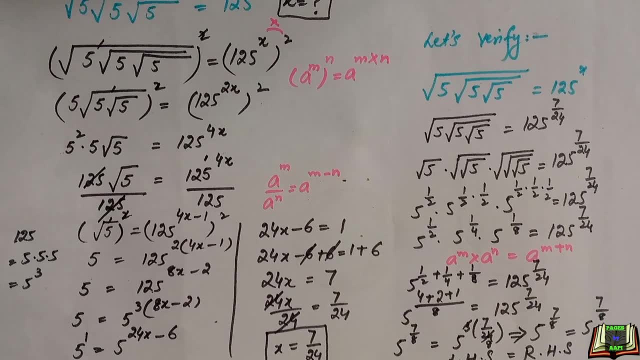 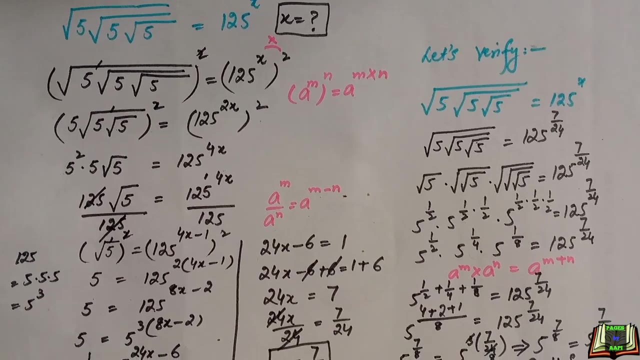 left hand side is equal to right hand side and it also means that the value which we got, X is equal to 7 over 24, is the correct answer. I hope all the steps are clear. if not, feel free to ask to me in the comment box. practice it and I will see you in the next video. 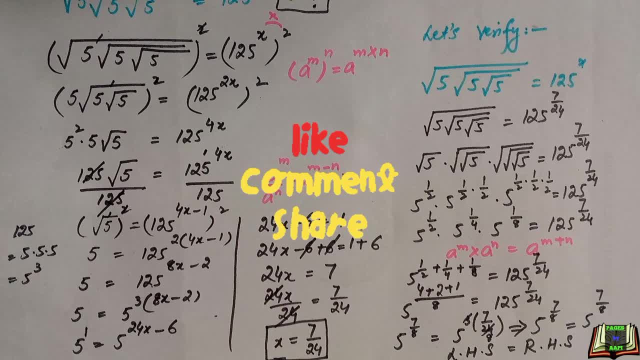 keep watching, keep practicing. don't forget to hit the like button and subscribe this channel for more informative videos. take care, bye, bye.